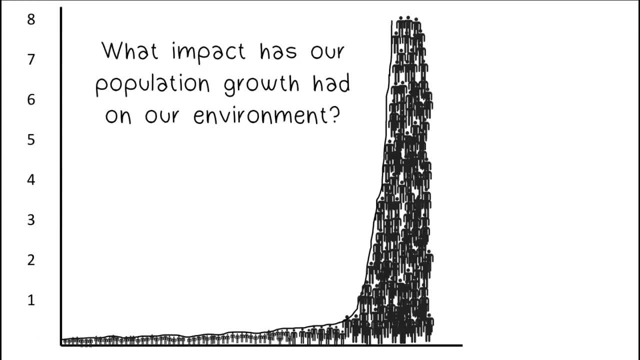 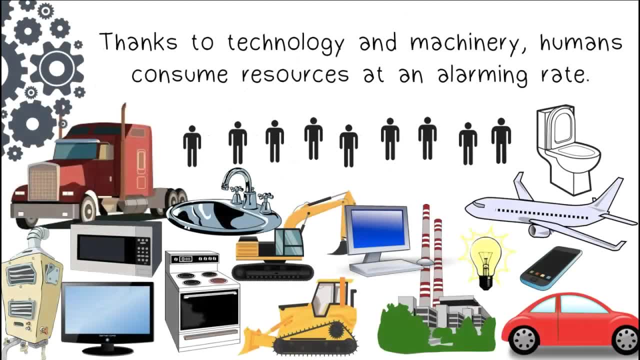 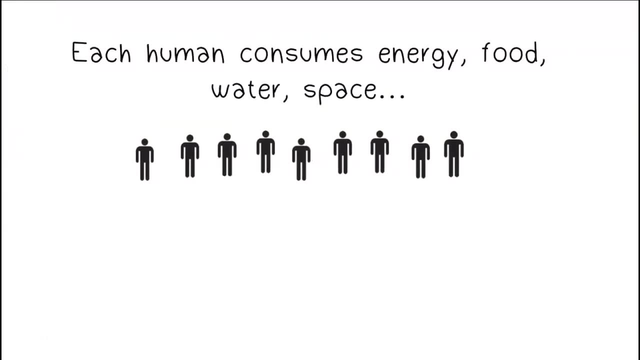 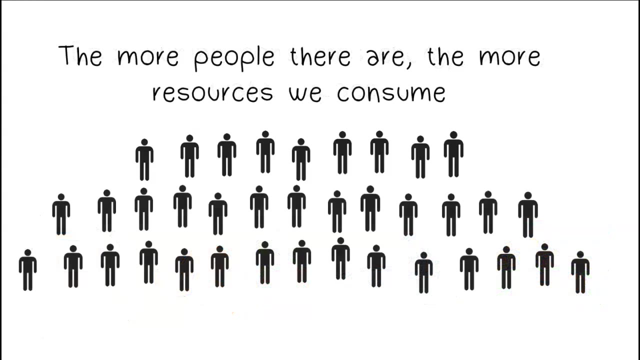 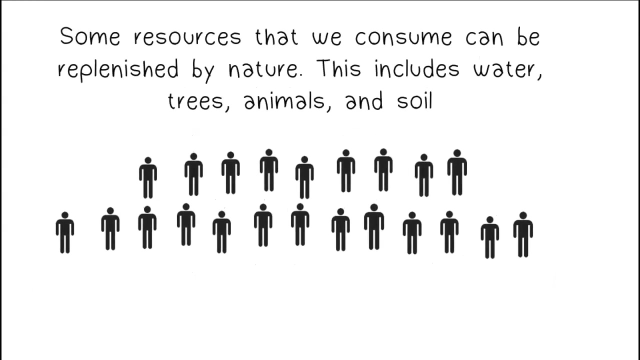 What impact has our population growth had on our environment? Thanks to technology and machinery, humans consume resources at an alarming rate. Each human consumes energy, food, water, space. The more people there are, the more resources we consume. Some resources that we consume can be replenished by nature. 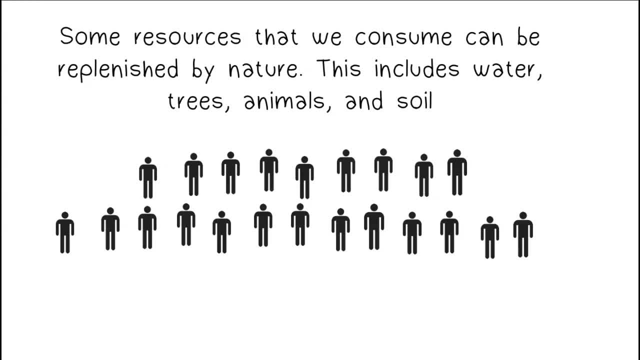 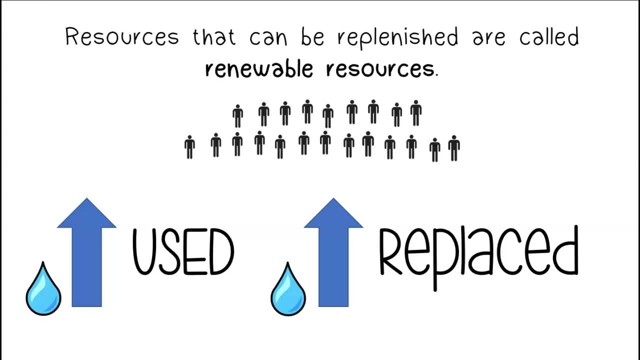 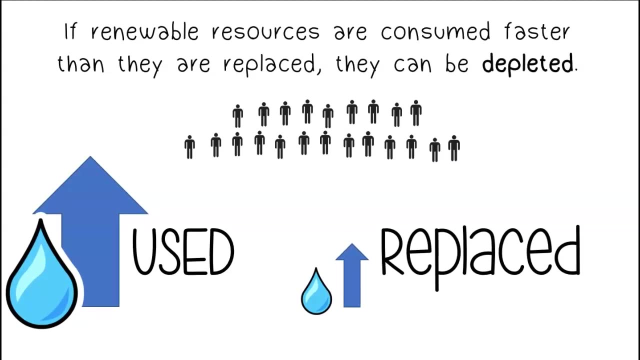 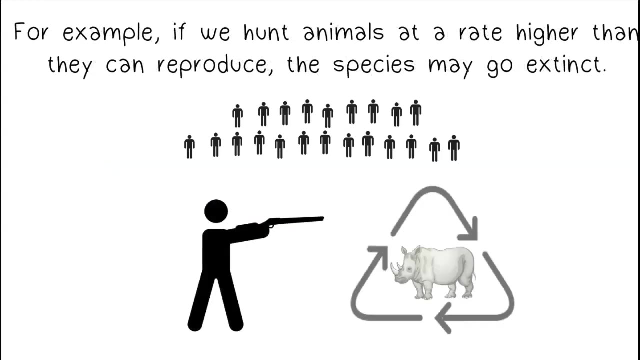 This includes water, trees, animals and soil. Resources that can be replenished are called renewable resources. If renewable resources are consumed faster than they are replaced, they can be depleted. For example, if we hunt animals at a rate higher than they can reproduce, the species may go extinct. 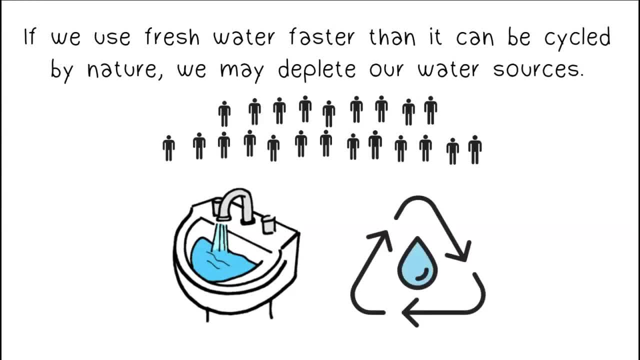 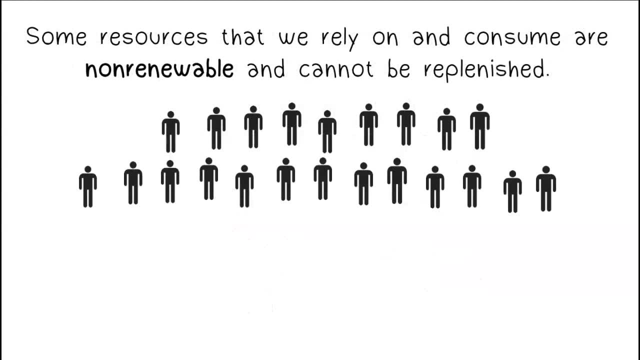 If we use fresh water faster than it can be cycled by nature, we may deplete our water sources. Some resources are consumed faster than they are replaced. Some resources that we rely on and consume are non-renewable and cannot be replenished. 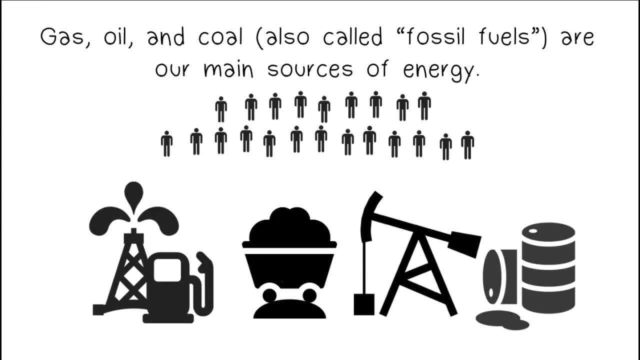 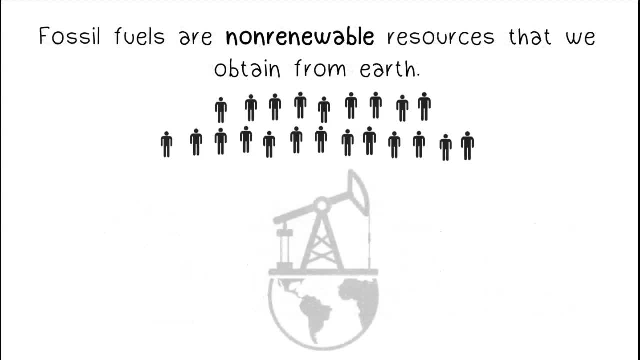 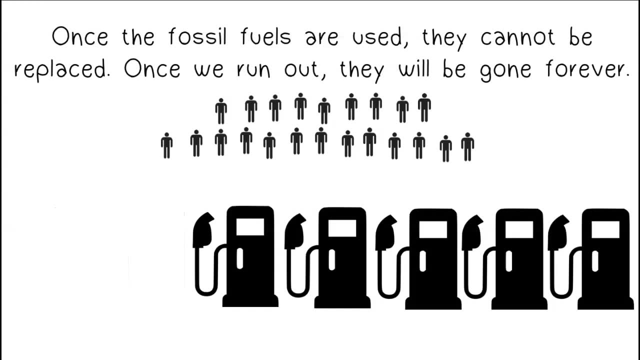 Gas, oil and coal, also called fossil fuels, are our main sources of energy. Fossil fuels are non-renewable resources that we obtain from the earth. Once the fossil fuels are used, they cannot be replaced. Once we run out, they will be gone forever. 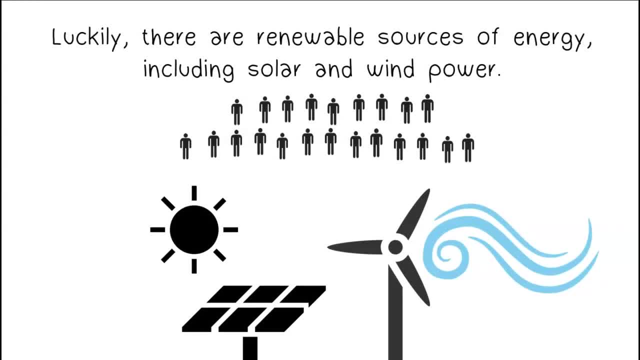 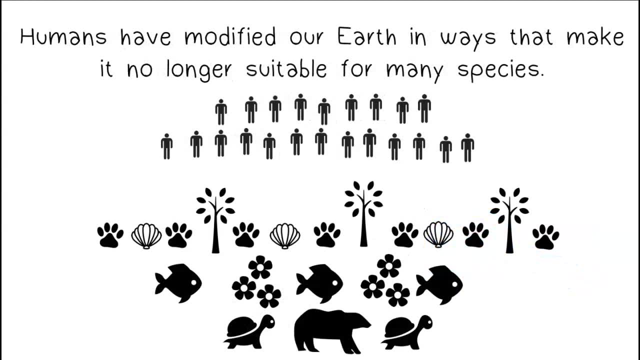 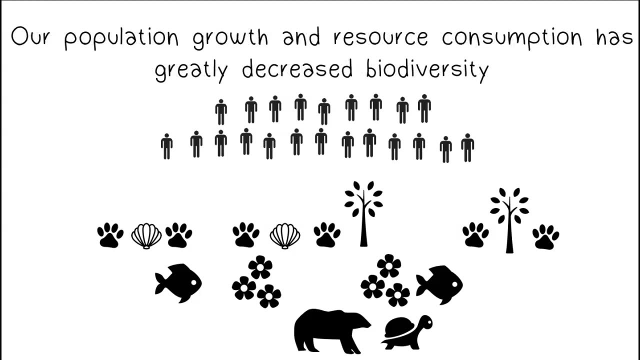 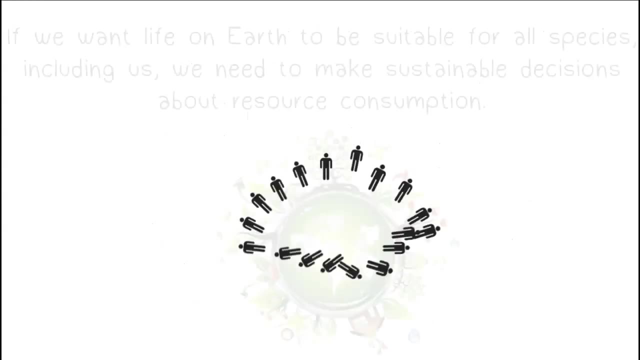 Luckily, there are renewable sources of energy, including solar and wind power. Humans have modified our earth in ways that make it no longer suitable for many species. Our population growth and resource consumption has greatly decreased biodiversity. If we want life on earth to be suitable for all species, 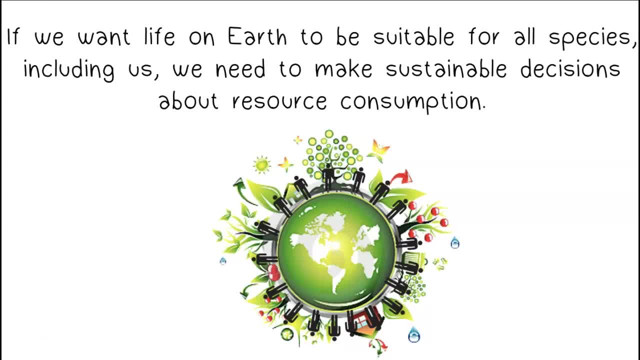 including us. We need to make sustainable decisions about resource consumption.